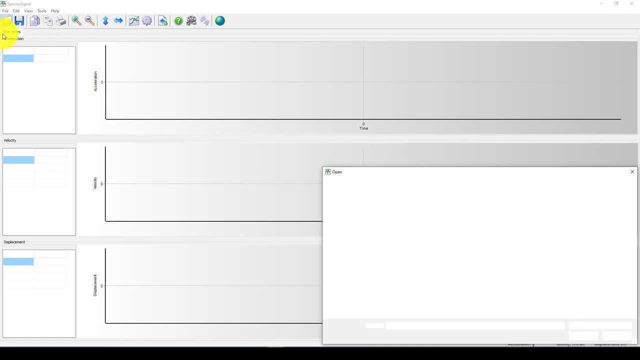 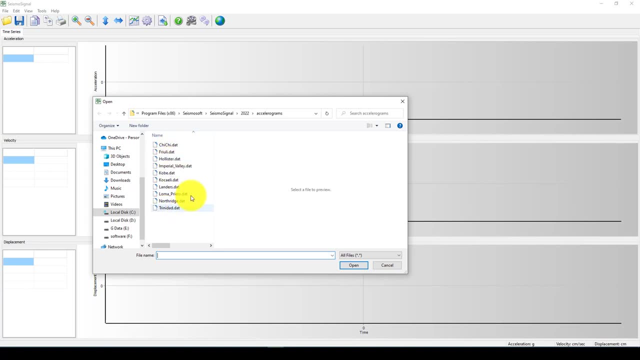 Some history analysis. If I go to open and you can see there is some installed Loma Prieta, Northridge, some TG and this also could be data. So, but maybe this is not enough. in some analysis you need at least 50 earthquake, 30 earthquake or more. So we want to get this data directly from the database which is already stored for that research. 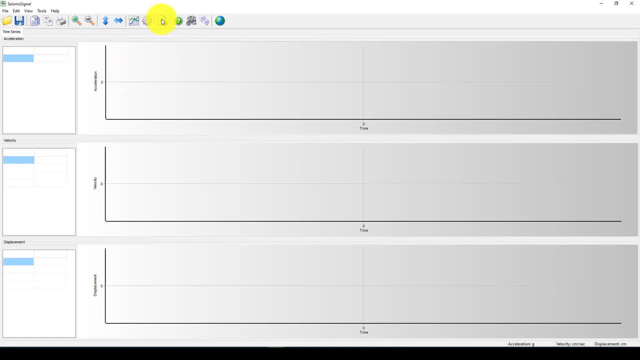 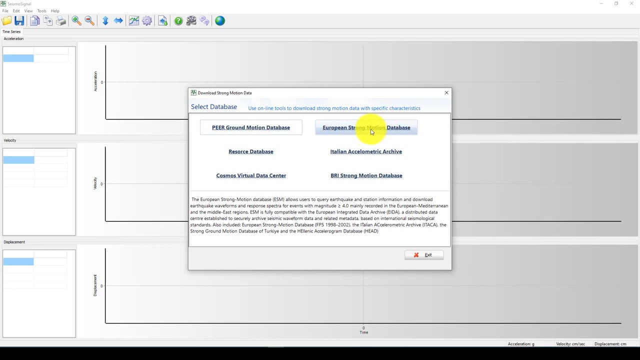 You come here in case if you don't have here, so I will show you both. So you come to the download strong motion and you can see there is six database. So the first one is peer ground motion database, which is the largest in the world, And the second is, like European strong motion database. I have access to some of them, But if you want to access to the European or Italian, you have to contact them by email and ask them to provide you. 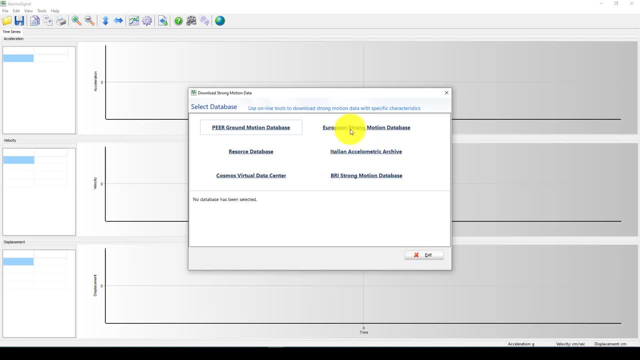 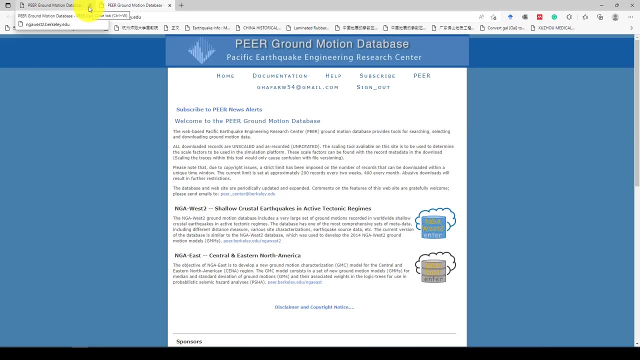 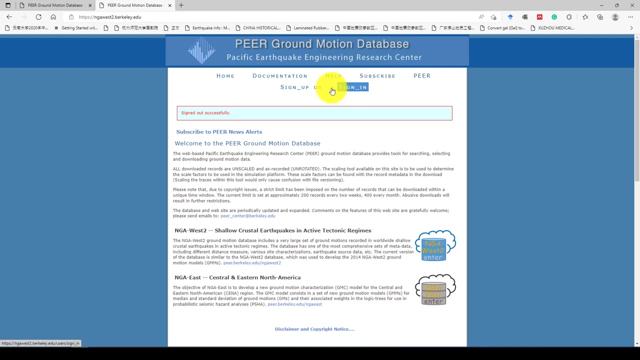 a username and also a password. then you can enter it down. It's a little bit complicated than this one. This one is totally everyone can, without contacting the administration. you can go there. So when you click here you will see this database. So you have to create, you should go to the here and you should sign up, So you should have an email address. 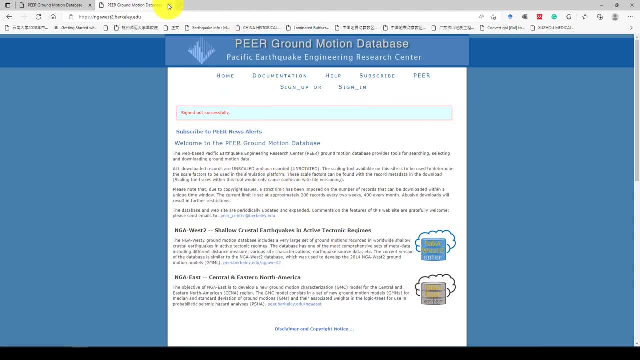 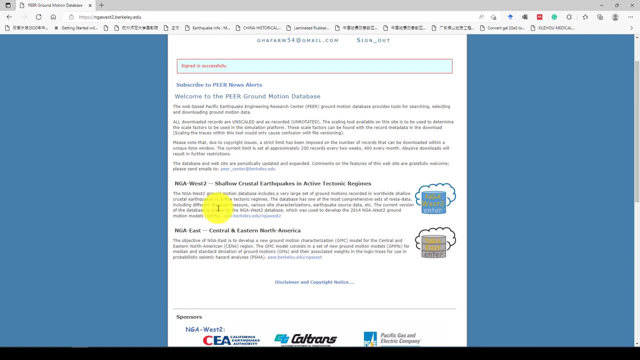 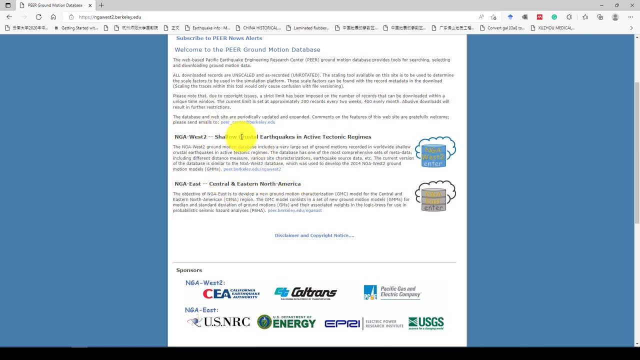 And then you can create a password and then login. So I have already and I can go to login. Then here is we have to talk to kind of database that one is NG note West, N食 West. So this is the central, is North American database And this is also the show crystal hard, quick and active technically'm region. So you canLL. 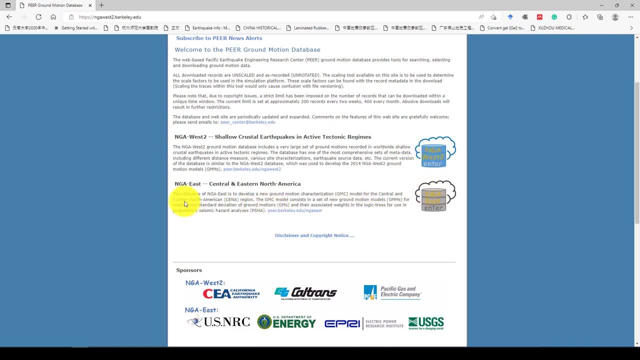 you can call both of them in case, if you need. and here is giving the information, Mostly these databases recording from where to where, data visit recording from where to where. So, for example, I go to that, this one, and after that you can. you see this pot and you can come. 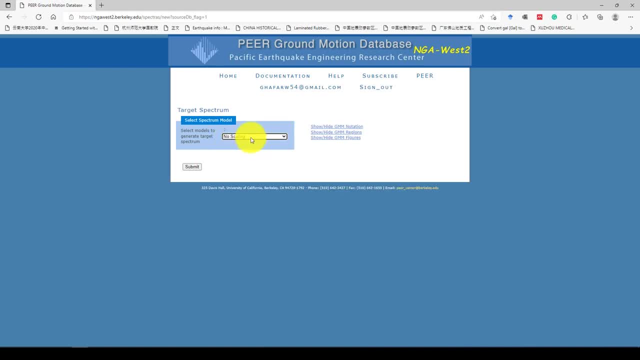 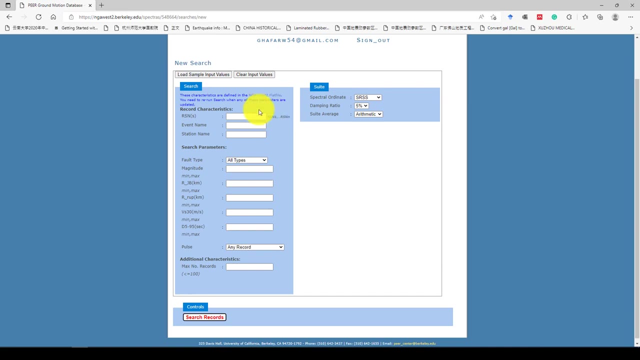 through here. so I want to get a noise killing, which means the exact earthquake from the ground recorded, but quick. so now here we will see the search option and you can give this one is a specific characteristic for that recording, like the event name, the station name or a same name. each country has this, this. 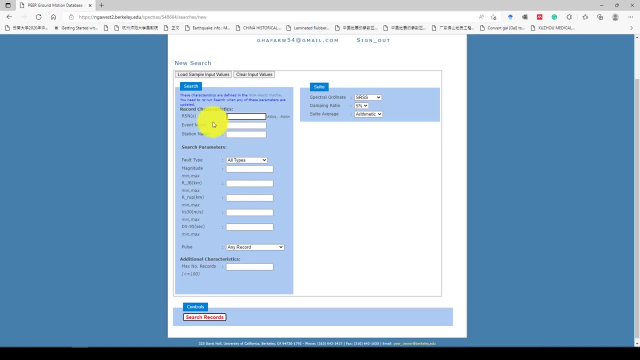 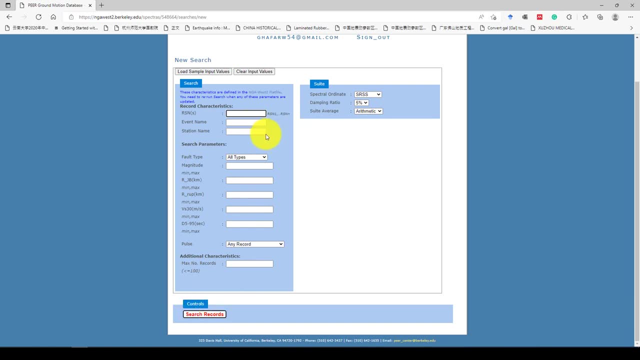 specification. so in case, if you know your country's specification, then you can give this exact number, name and you will just go to search. it's called the search report and you will find for you. but I don't remember none of them, so just I know that one of the very popular event 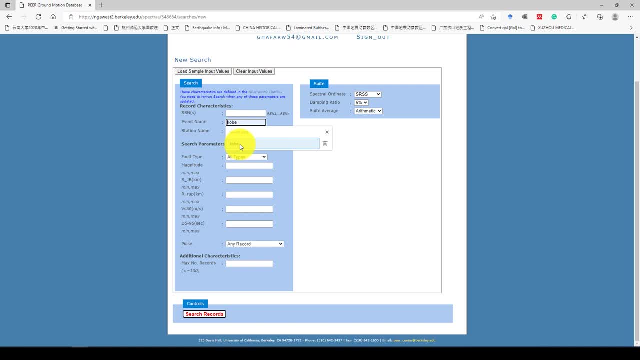 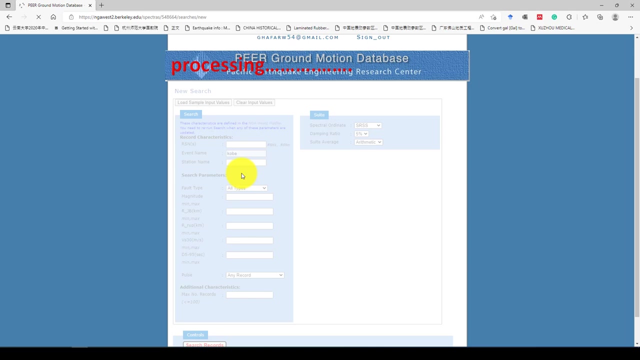 could be. could be or not, rage or bomb. bomb is a running earthquake. this is very popular and it's very catastrophic earthquake in the world, so that could be is also so, just like he gave the copies to, in the copy name there is will be thousand earthquake recorded. so I'm gonna call search and you can see this. 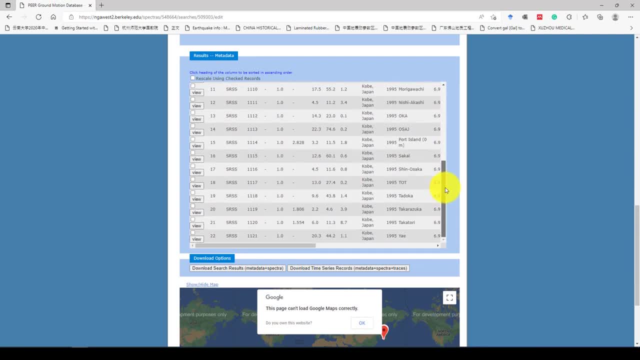 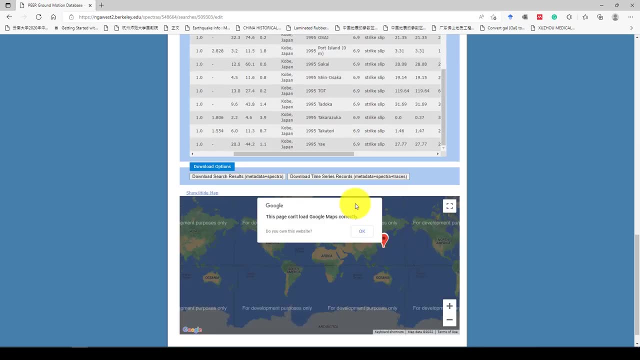 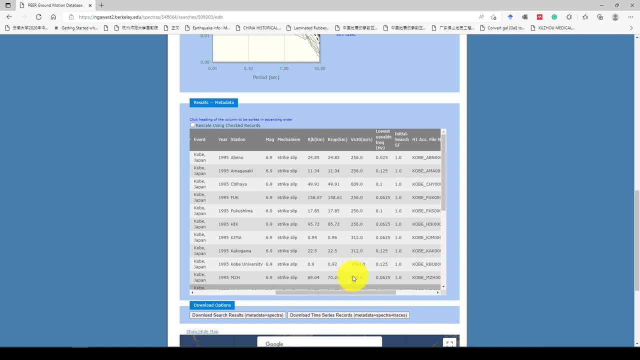 record is visualized here so you can see the most earthquake is over nine, over six point nine, almost six point nine, and you can see the sort of earthquake, the mechanism and also the location or the epicenters and also the ruptures and velocities and all information is giving. so what we're gonna do is you can, you can use this. 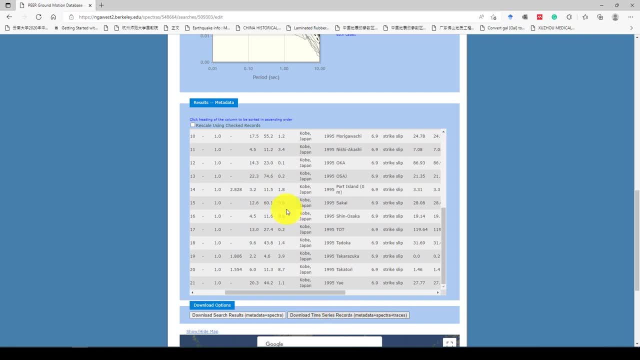 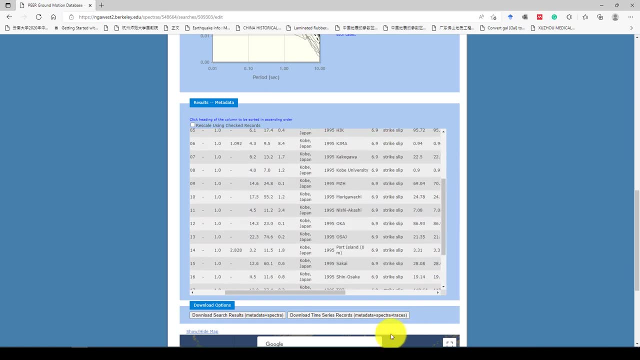 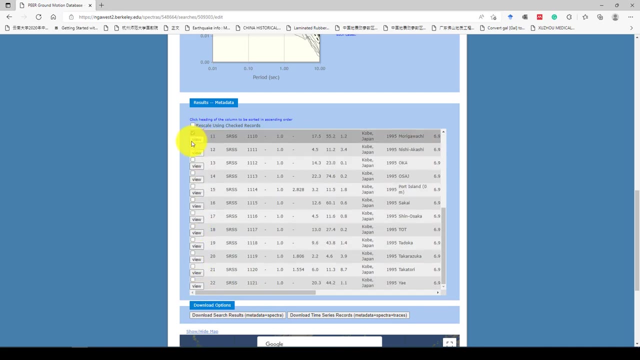 function is here: download time history record. if I want to re-scale and go back to give some scale, make one point two. so there's no need because we need another application that we can use it. so in case I want to go to check one of them or see, let's go. 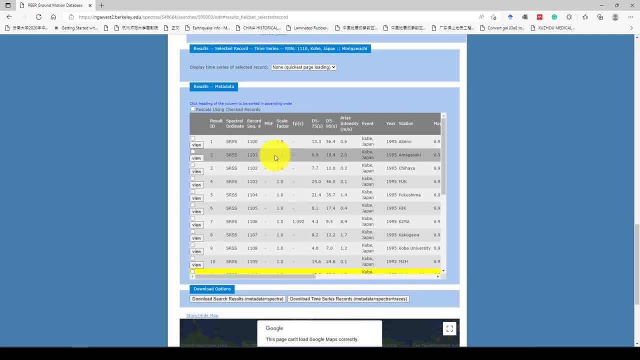 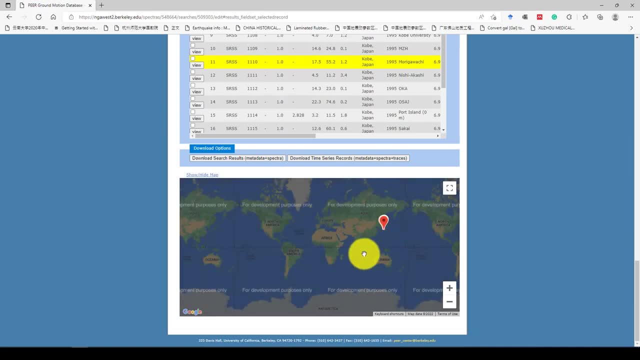 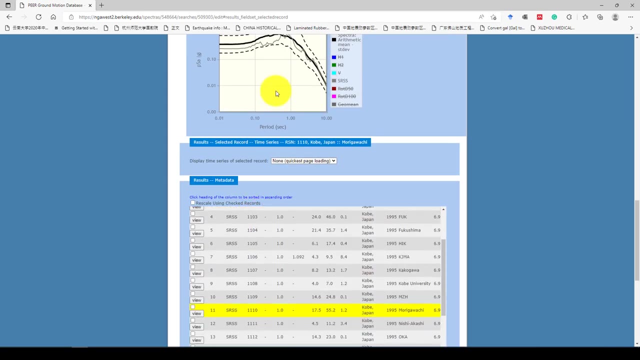 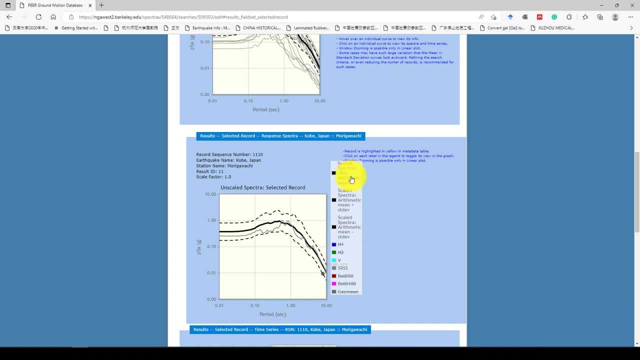 to view this one and just now, instead of using all them, and we selected one of those one and this is the location. this is a location of that earthquake and also we can see the graph here. this is that you can see. you see the spect" www. 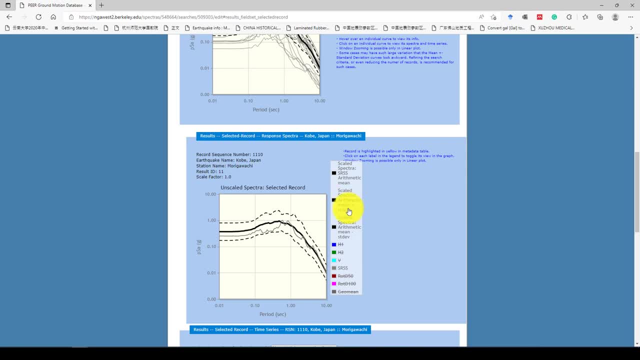 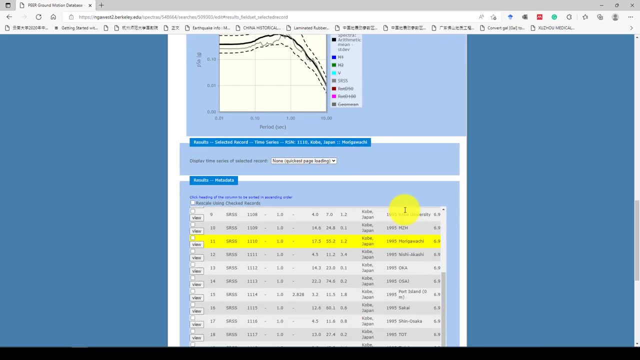 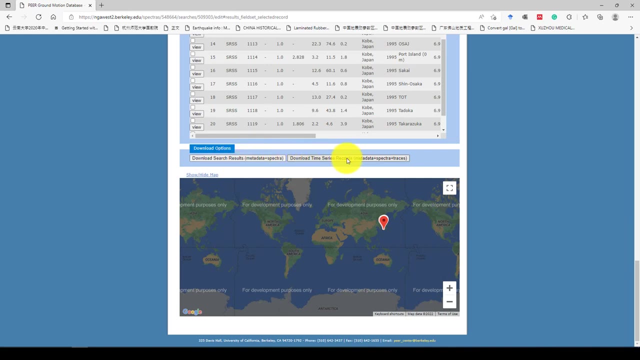 graph we just showing. there's spectral spectra, hol, 맡ixinas and also spatial. so this is so. we have this too, And then we can go to download this one. You can consider download search using metadata spectrum and you can download time series. So I'm using time series, I'm going to call you have downloading this one, So automatically it will download for me Just take a while and then it will convert into the zip file. 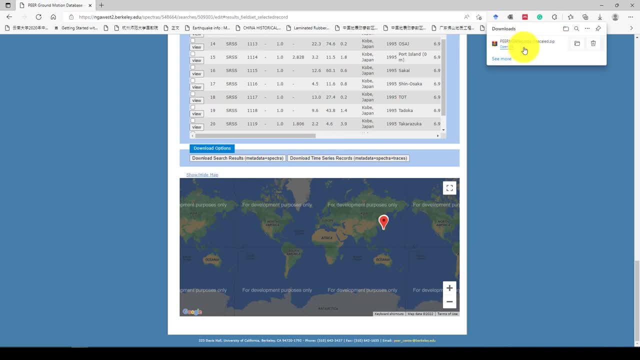 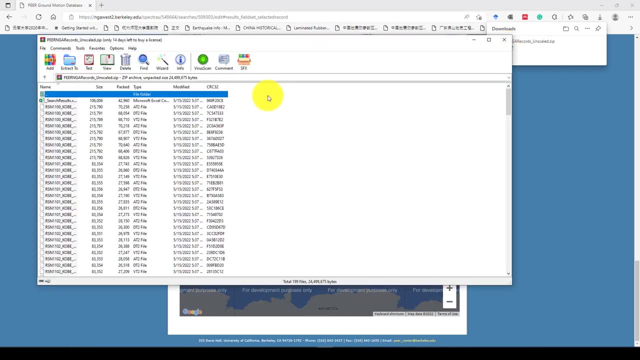 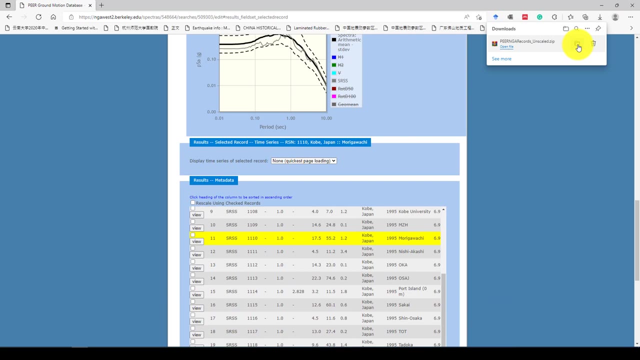 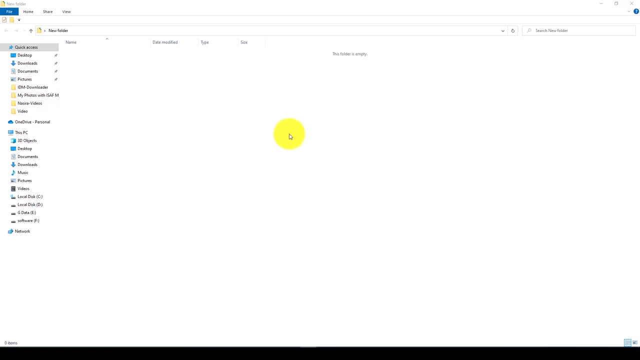 And yeah, here is the, the program, because if I go to the that file, go to open, I can go to open file and here is the giving data. So if I let me go to first that that area, and I'm going to let me cut this one, So I can't cut it and I'm going to paste here- 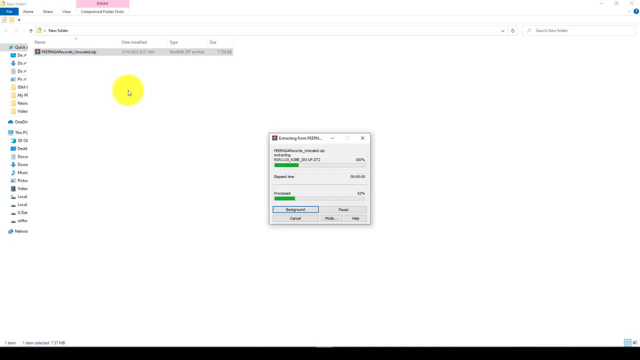 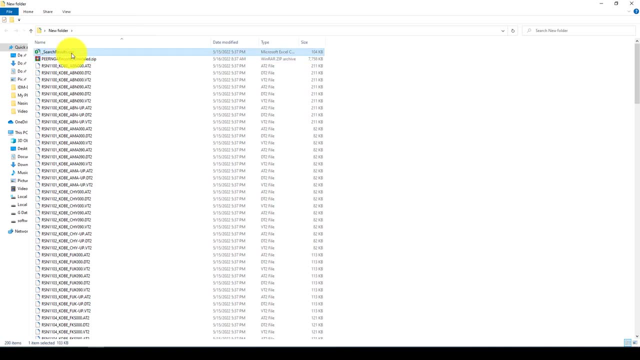 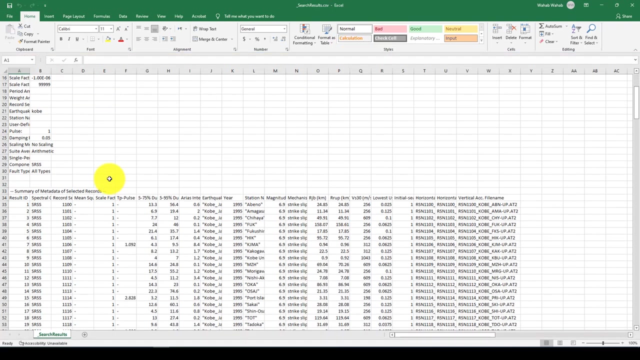 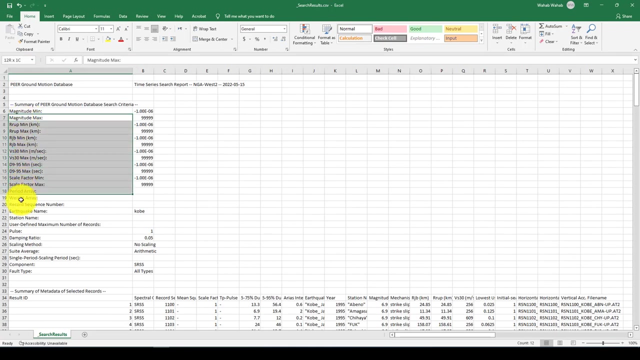 I'm going to paste it here And I want to unzip, extract And you can see all the data is giving. So this data is giving some specification. Let me open the CSV file, or Excel file, And you can see. now this is the first information, This is the information. you can read the exact location, raptures, everything from this one And also consider the dumping ratio. 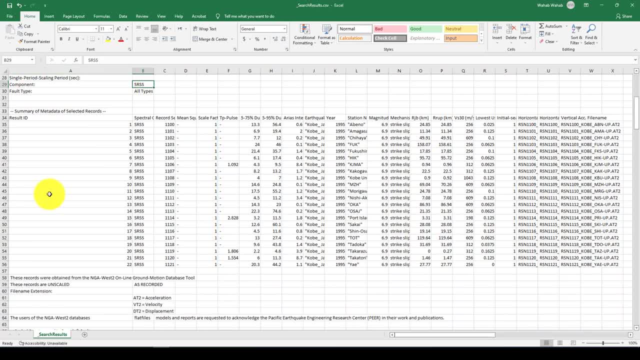 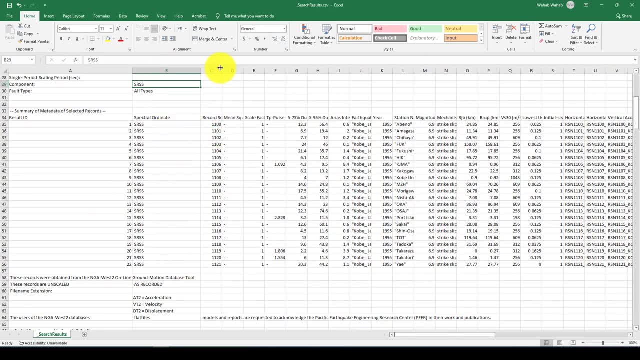 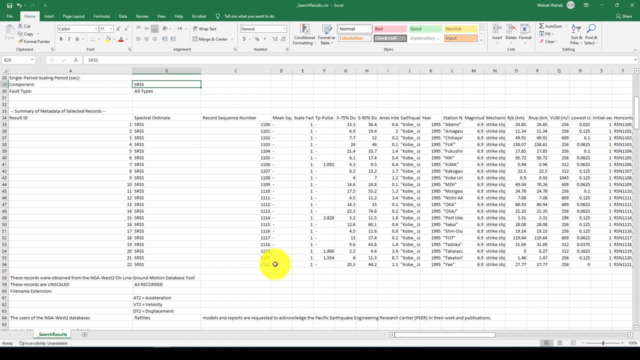 χ To unpack. that Allez goes more to. now you haveningar, don't you just drive? and all that automatic. This is giving another information. This is called the coordinates number. So we have from 1000, 1100 to 1000. 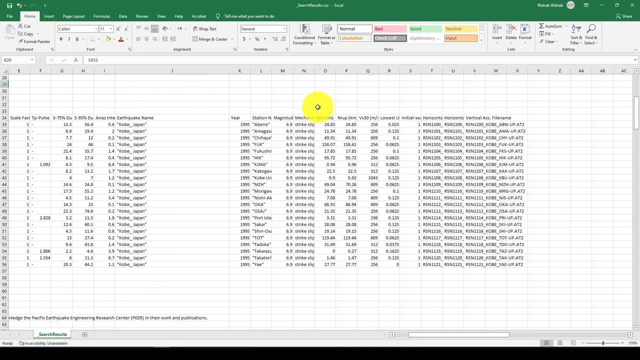 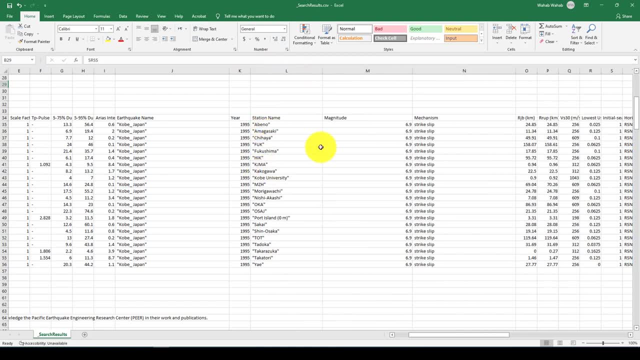 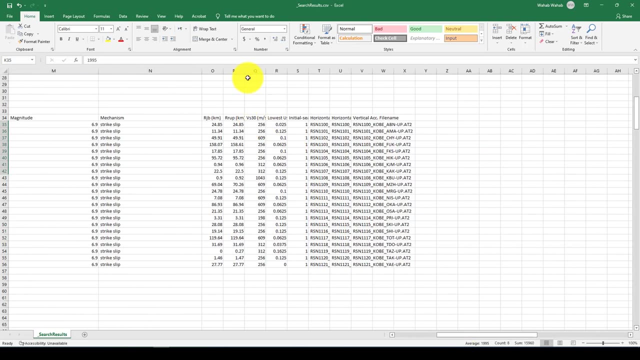 So�� apples 20 mann record it downloaded, Don't know, you can come straight here. Um, among the Oh, no, no, no, no, no. magnitude of the earthquake and the location: this in the station name and the year which this earthquake is occurred. and here is the. this is the. 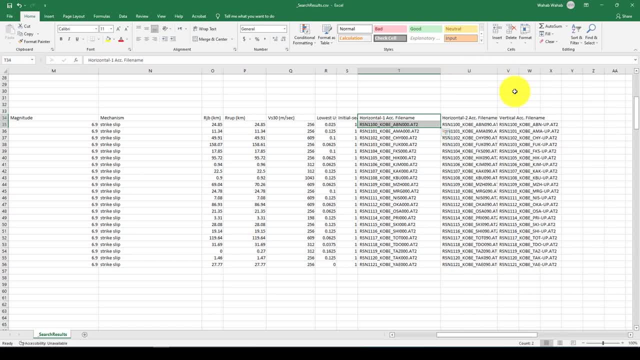 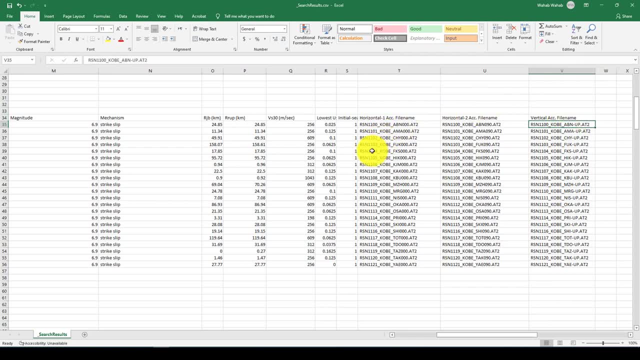 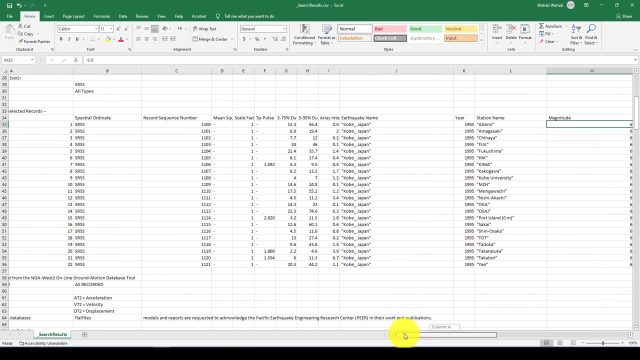 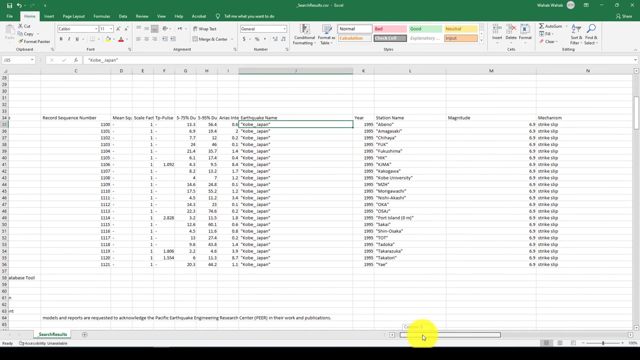 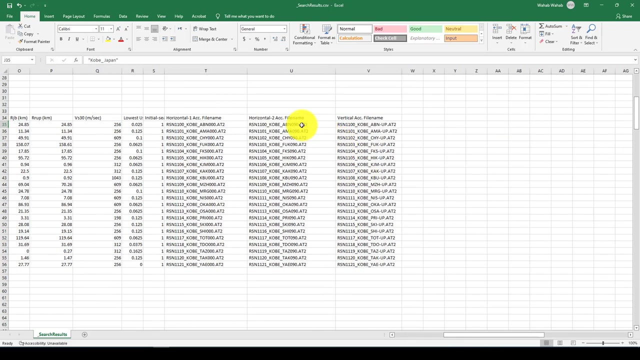 horizontal acceleration and this is also the vertical acceleration and the name is giving here. so now I want to see the horizontal acceleration of this earthquake. so this is a quick, this desert quick did the first one. so it is in a vino in Japan and it's 99 and the magnitude is 9.9. so I want to get the. 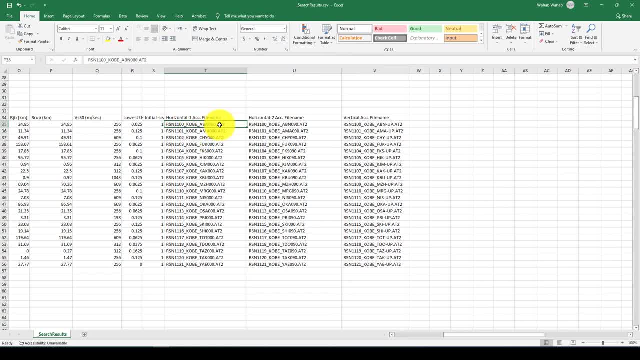 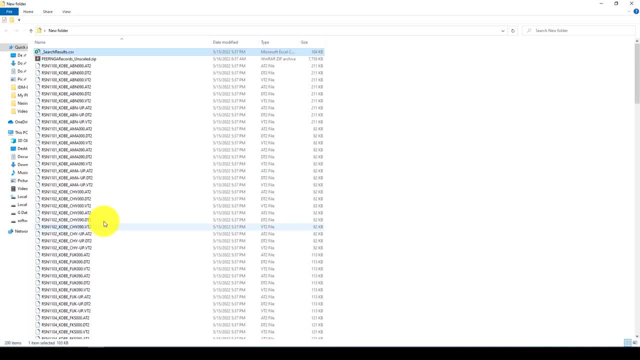 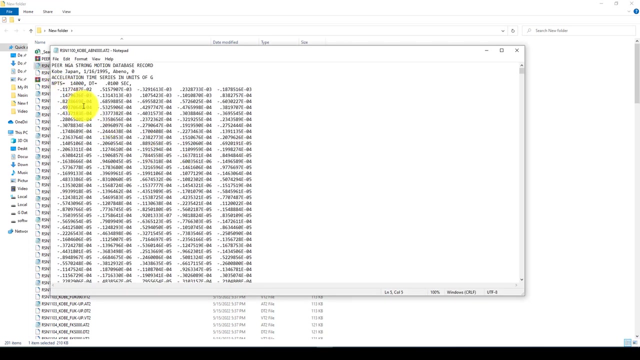 horizontal acceleration. so this is the first one, is the horizontal acceleration. the a tu 282 and I'm gonna go back to here. the first one is 82, so I can open in automatically to that text file. open with, open a text file and you can see the data is like this and it's a copy-john. 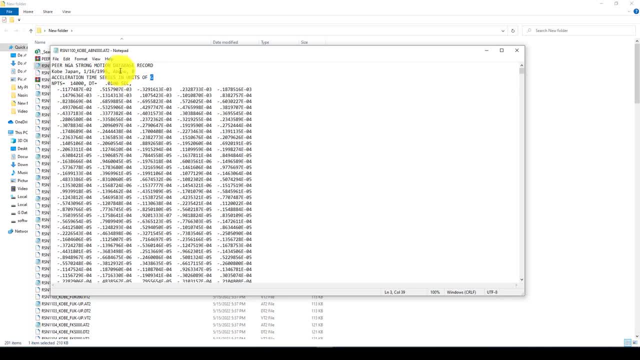 copy-john upon and exclamation time. the unit is G and the name is this one: 99 years, and the total number is 340 thousand. and stupid, between each record is 0.1 second. so what we're gonna do is I can upload this one to my software and I can go to. 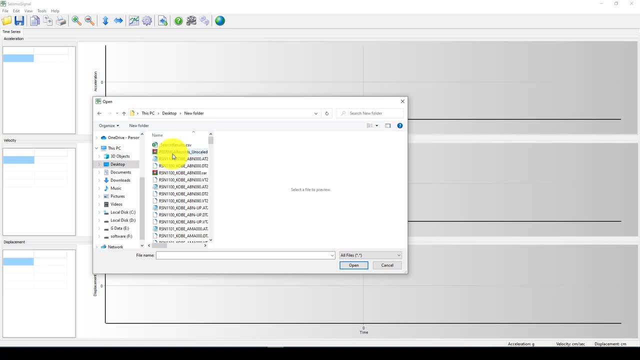 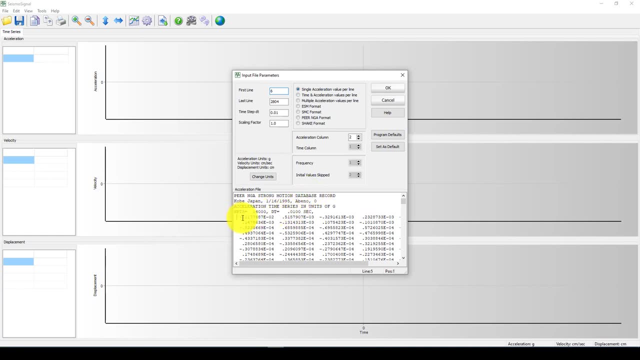 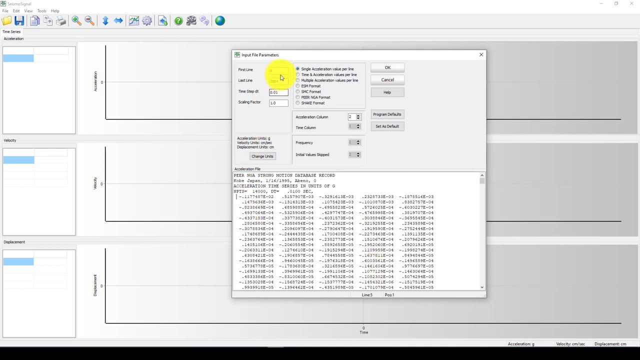 open here and go to the desktop and here is a new folder and the first one was my 82. I'm going to open it and I'm going to see the data and I'm going to see the. And you can see I should give this information to the software. So the first line is here. I posted line 5. So it means first line is in line 6. And the last line is be about 15,000. Because it's 40,000. So I can give it 40,500. And the data time is giving this one 0.1 second. The scale factor is not scaling. In case, if you want to scale, just give 1.2, 1.5, as much as you want. 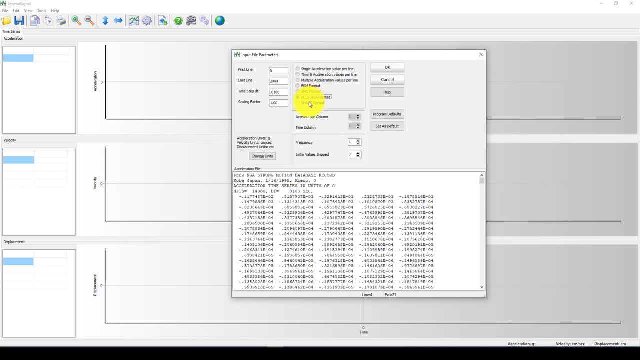 And now here is called peer ground. You can select this one, It's automatically detected this one And you can last line: is Okay, this one, And time step is this one And I'm going to. The unit is g And we will see the velocity in centimeters per second And displacement in centimeters. I'm going to, okay, And you can see the record is created. 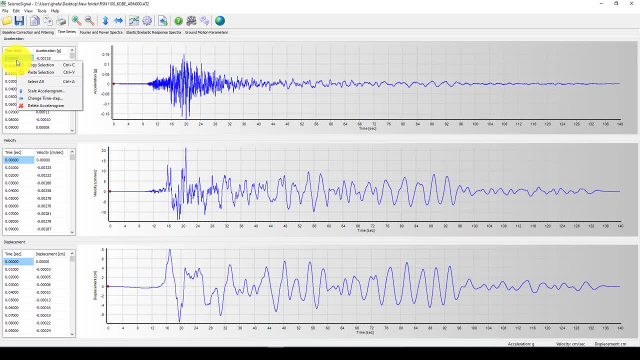 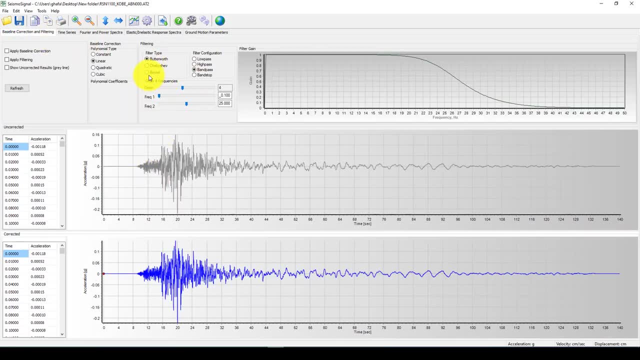 Okay, So like this, you can then select for your analysis And you can use this one, And also you can do some filtering or some sort of using some filtering, Some sort of correction, And also you can. You do not need to use this one. This part is very short. You as well as you can cut this one and you may reduce the time periods. 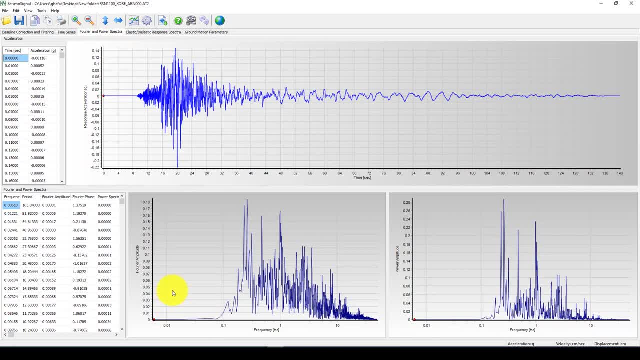 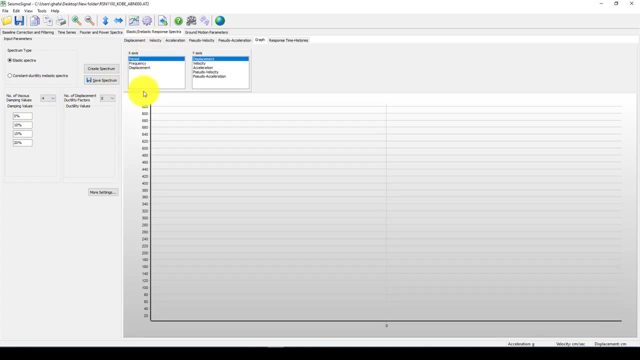 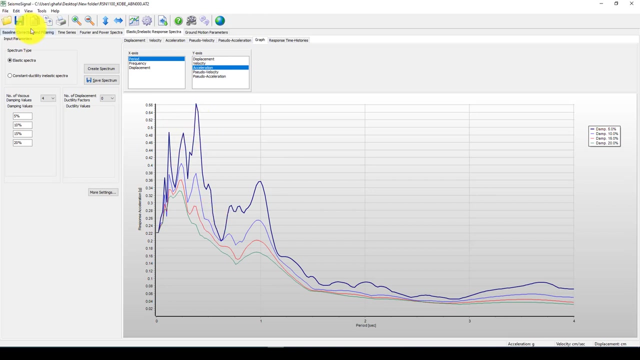 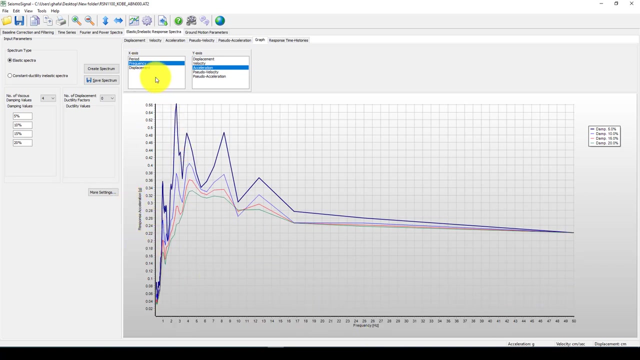 And also you can go to here, Use the For your transformation method And using this FFR And also you can get to see some, Create some dumping And also let's create a spectrum of that curve. So this is now giving time histories, response spectrum, And you also can get the response spectrum by frequency And also by displacement or C2.. 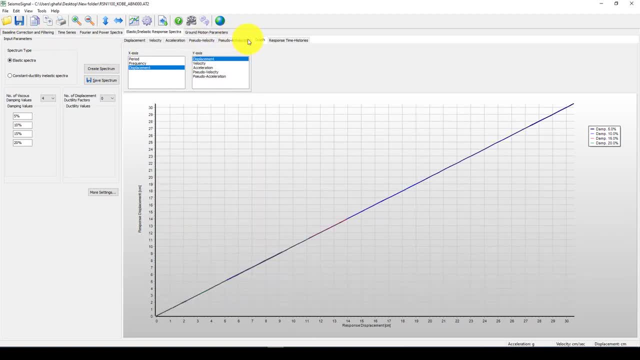 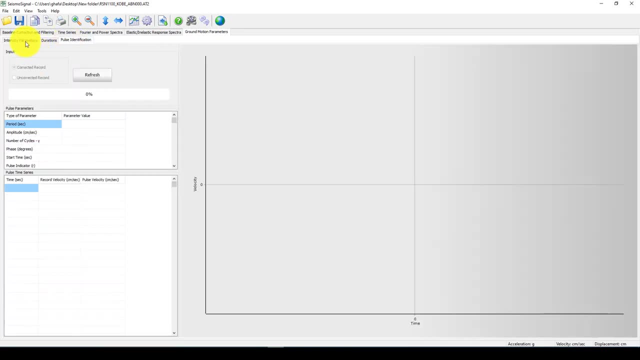 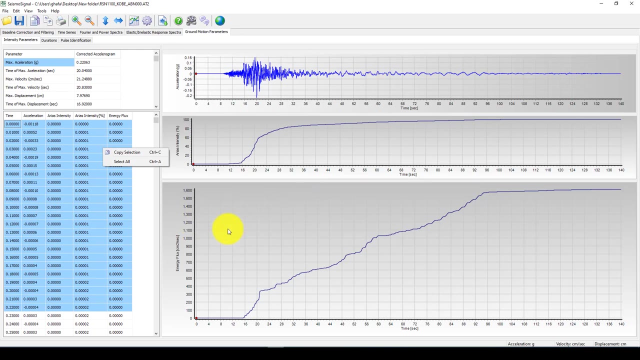 This Curve And for the last one You can just go to the ground motion parameters And you can come, Just go to the here And you can select all of them And just go to select all And copy selection And paste to another text file And then you can use for your work. So another way is just you give this name. 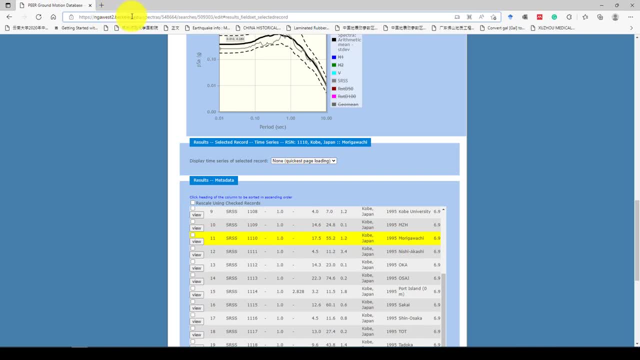 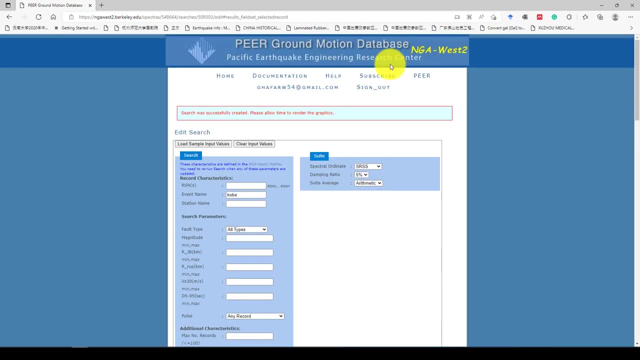 And you can give NGA West or Berkeley University. You can go to this website and Get this, This data. Then you have to create a account And then you can see. You can download any record you want. So this is the end of the tutorial. If you have any questions,